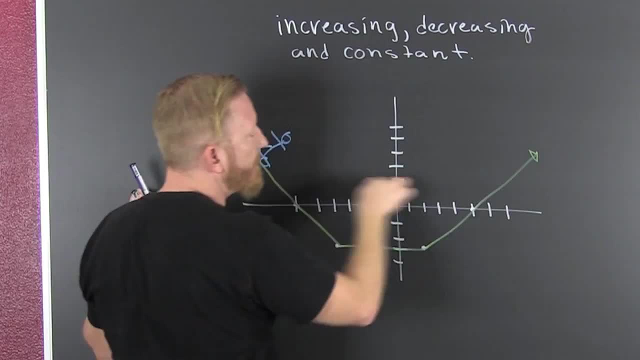 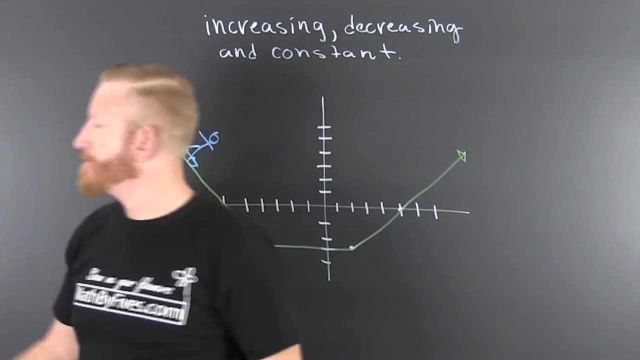 say World star? No, If you're going from left to right, you want to know whether or not you're going from left to right. If you're going from left to right, you want to know whether or not you're going down, down, down, down or up. Yeah, Sure, I don't have a tech. 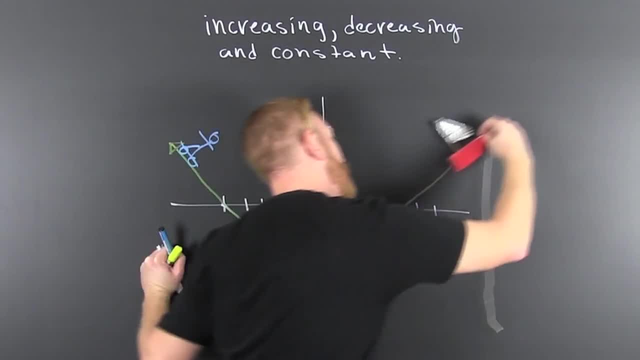 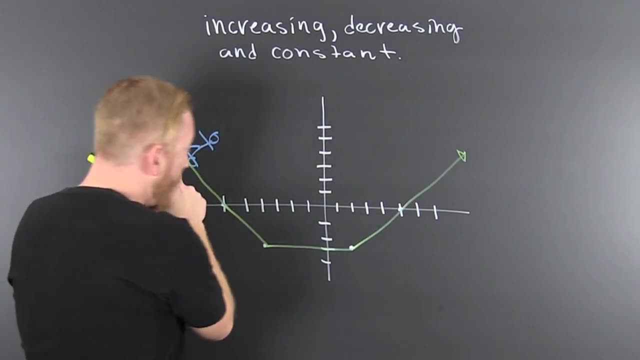 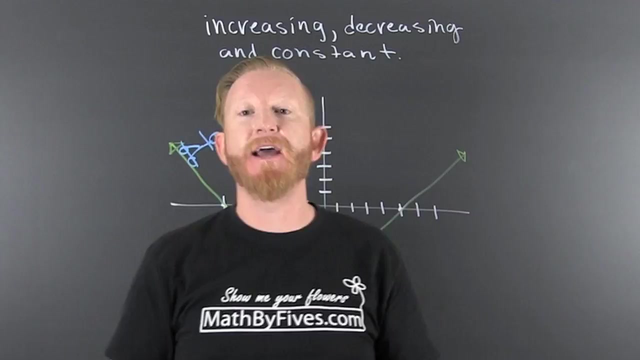 deck, but I got a little boat. Oh No, style points on that. I think I broke my boat. What are we trying to do? We're trying to see whether or not this is going up or down. So then, when we're going from left to right, we're talking about the independent variable X. 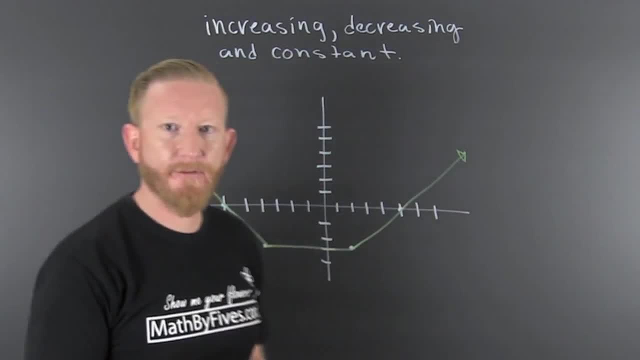 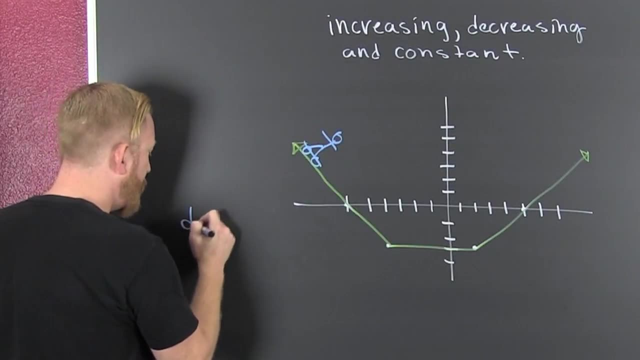 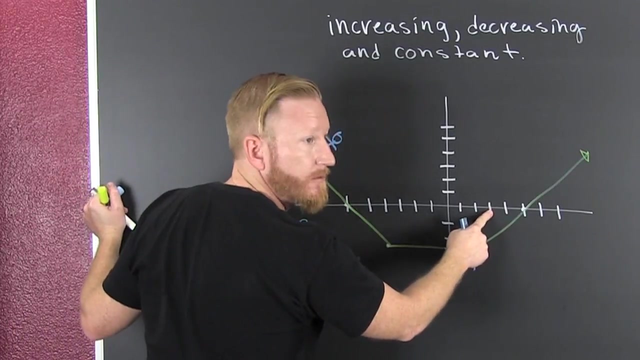 X is making the function do stuff. Yeah, Sure. So we are going down from year to year, So we can say we're decreasing D-E-C-R-E-A-S-I-N-G on which values of X, These values? No, Those are going up, These values are going down. 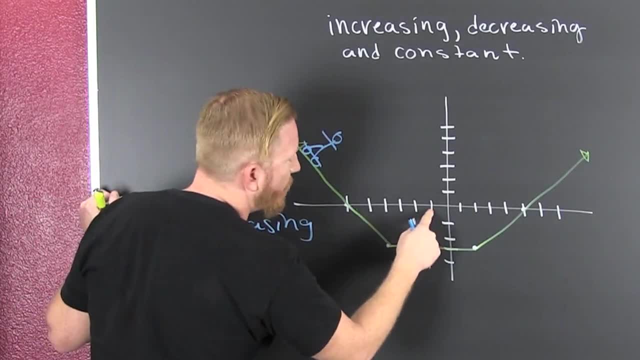 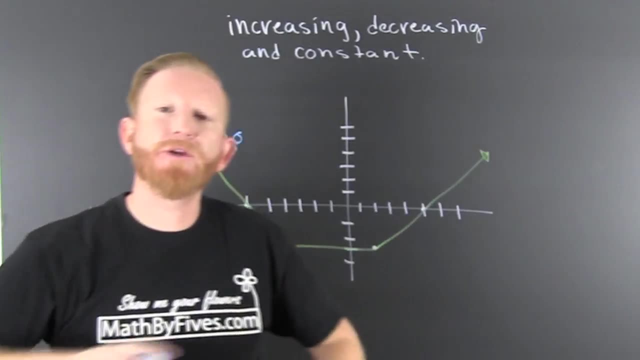 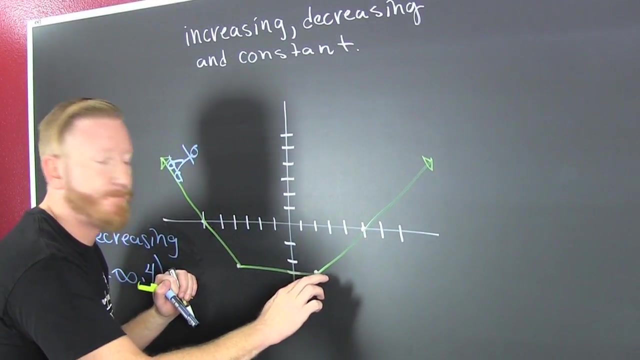 So that's minus infinity All the way to where One, two, three, four, Boom. Minus infinity to four, Sure. So what's this constant? The constant's where you have no change in your function. No change in your function, Meaning that you cruising along there. 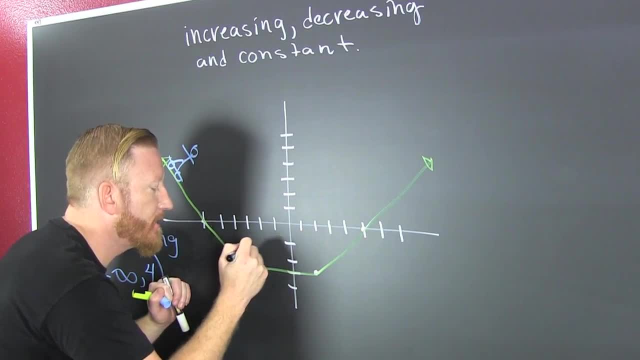 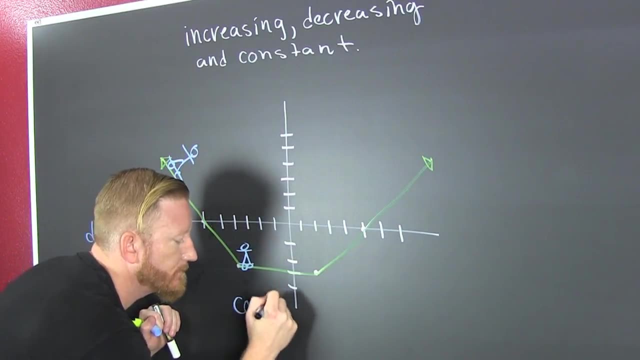 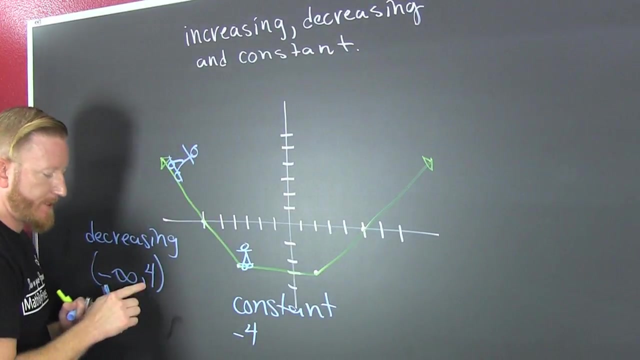 You're going constant Boom. Resist the urge to get your tech deck. We're trying to learn math, So we're constant. on what values of X? We're constant from minus four. well, that should have been a minus Relax. 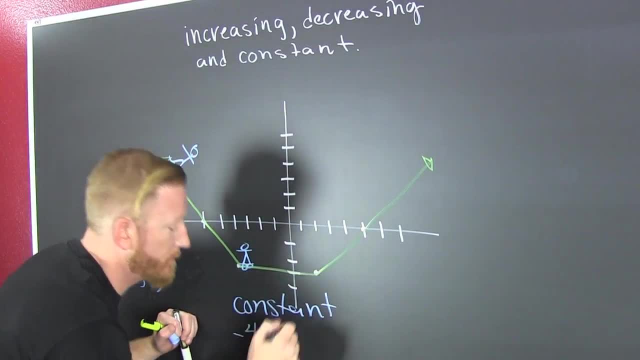 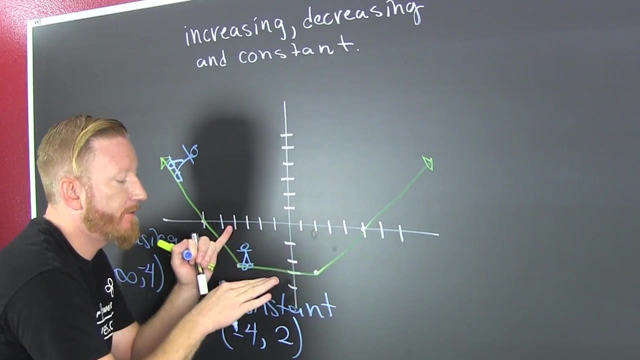 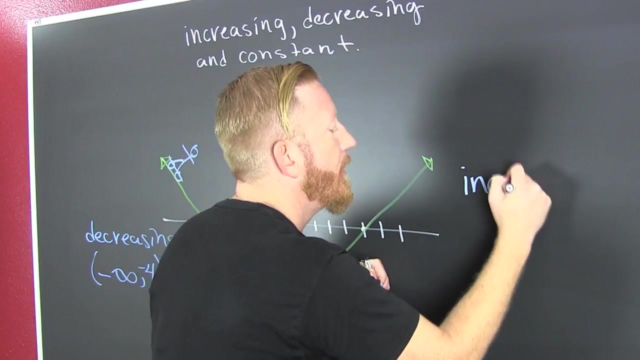 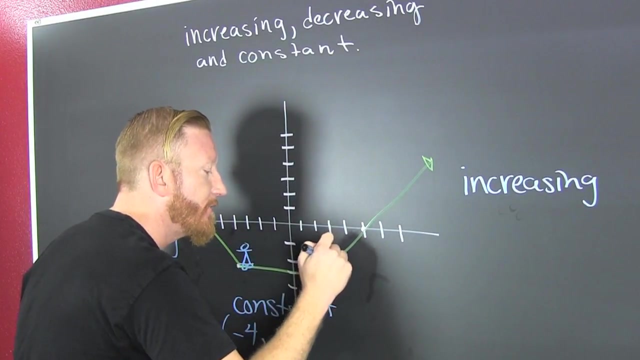 Relax, Relax, two oh two, oh. so then you're constant on that interval because you're talking about which X values keep the function level. so on the next level, we're looking to see where it's increasing. increasing the function is going up if you're going. 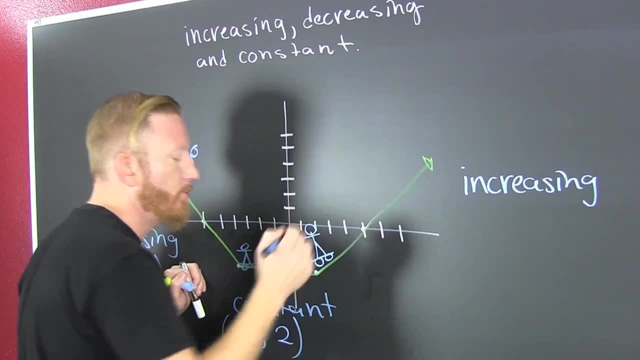 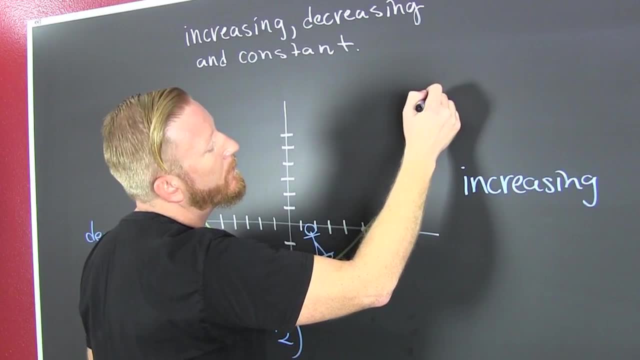 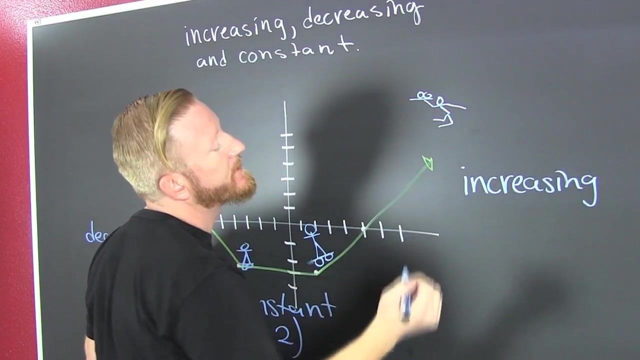 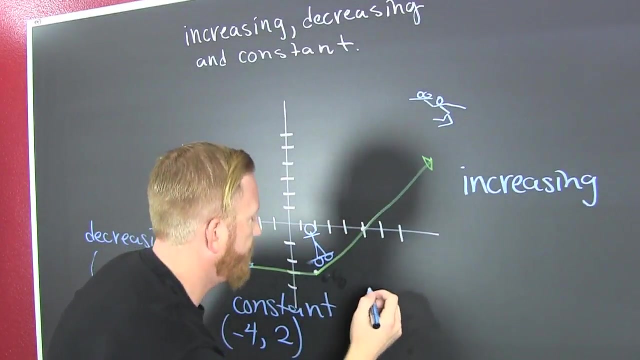 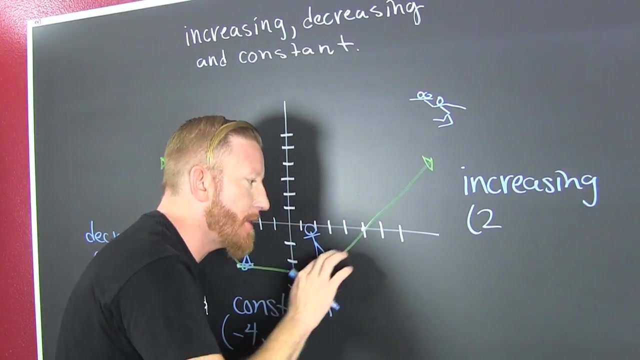